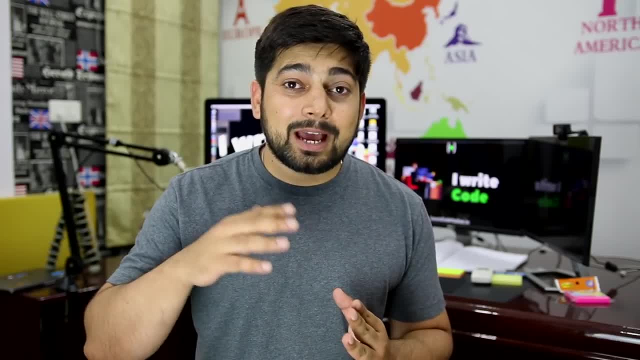 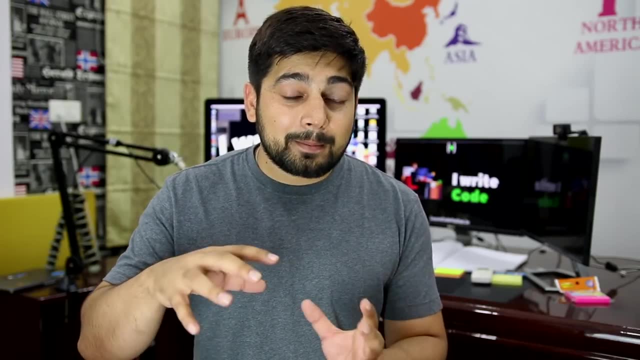 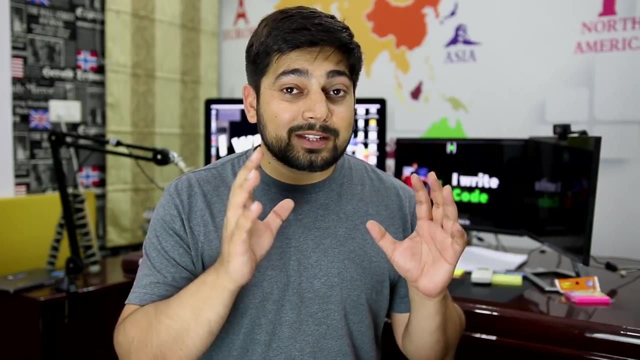 one of the most used databases on the planet. So many applications already have been designed in it and are still using it. It's amazing- and also when I say the term- that compared to relational databases, these modern NoSQL databases can perform really fast. don't get me wrong about there, because 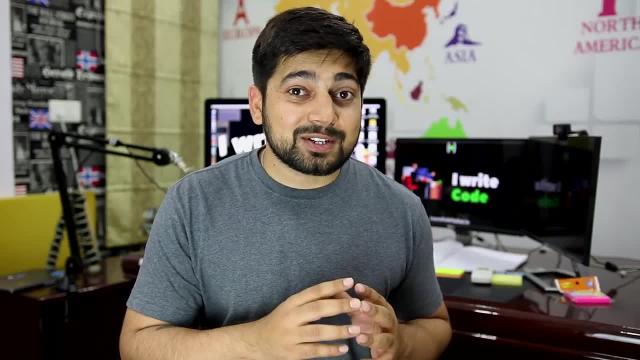 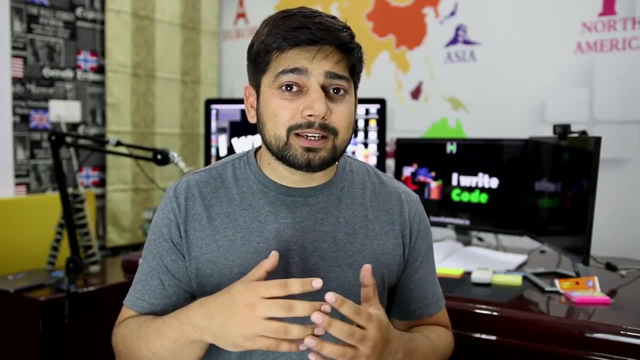 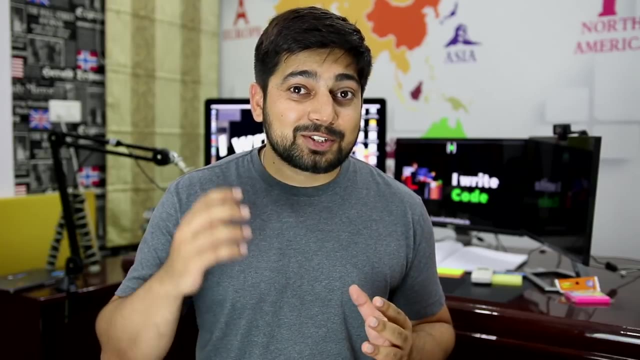 these relational databases can handle thousands and thousands of queries in just fraction of seconds. But what we are talking about is not the queries that you and me are making for a small scale website. What I'm talking here is about these gigantic website that throws billions and 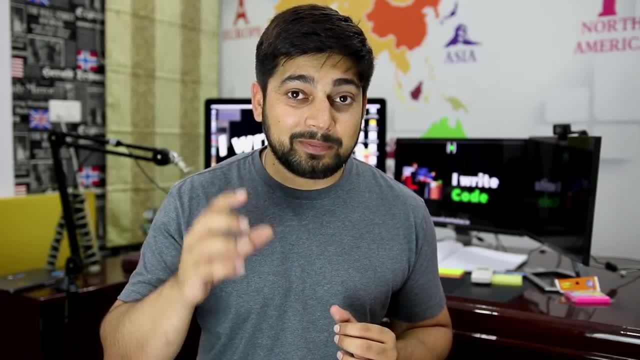 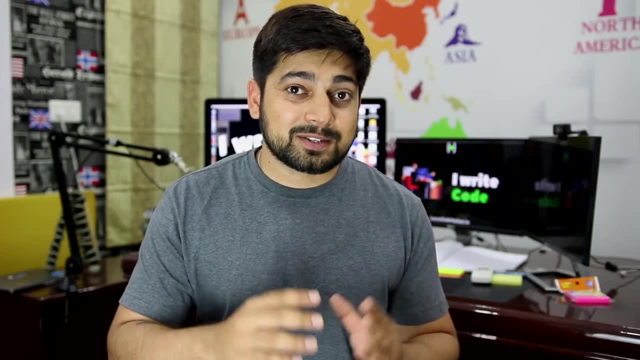 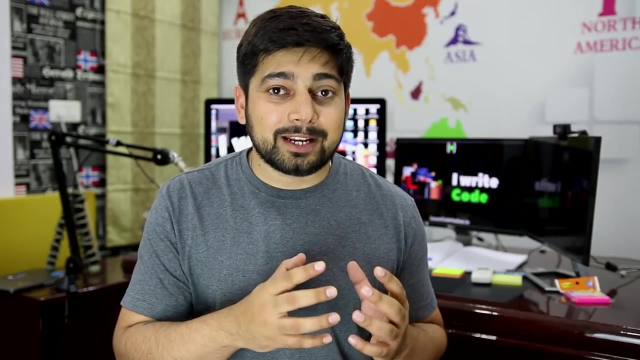 trillions and gazillions of queries within a small amount of time. Websites like Facebook, Amazon and Google. their transactions of these queries is innumerous. These NoSQL databases actually arose to get rid of some of the limitations that were there in the relational databases and mainly for 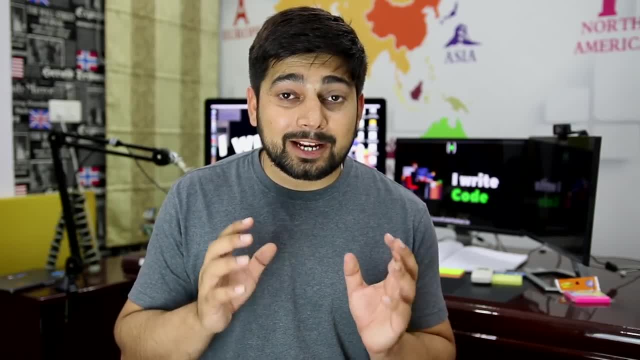 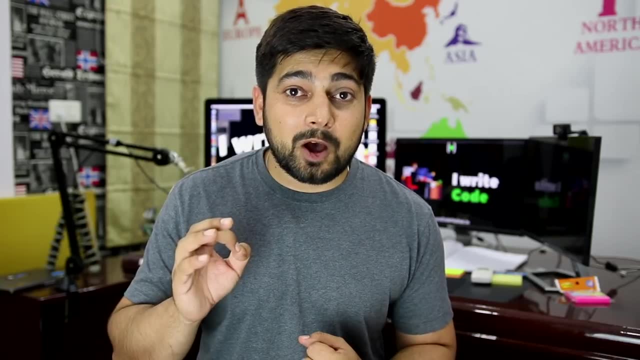 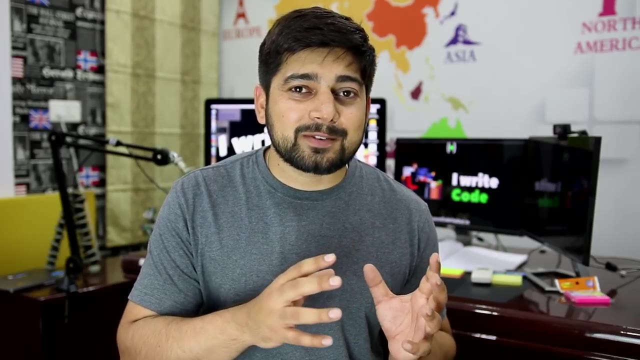 a number of reasons: First, high operational speed, and second is flexibility in storing the data. Yes, there are many other features in them, but these two are the most common things that gave birth to these NoSQL databases. Now, most of these NoSQL databases has been founded by these big 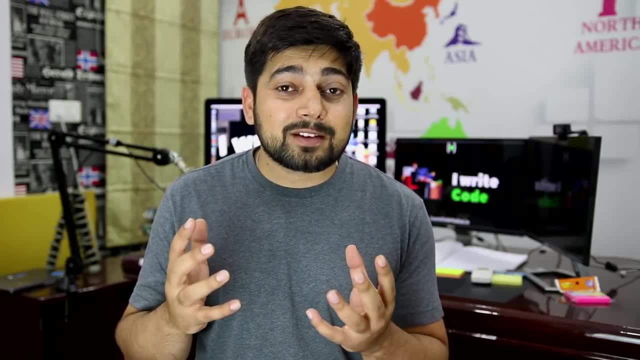 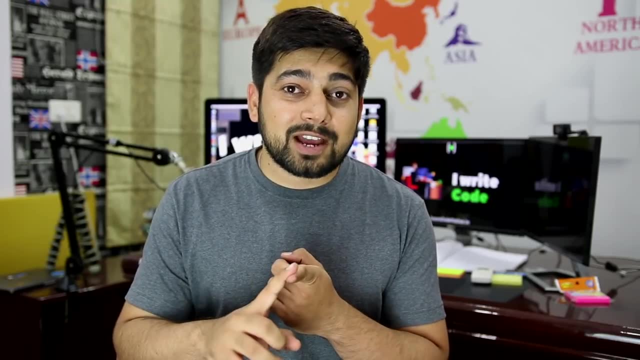 companies like Amazon, Facebook and Google, because they, first and foremost, felt the need that there should be a database that should be following these two practices: High transactional speed and flexibility of data. Now, here's the one thing which I would like to point here Now: relational. 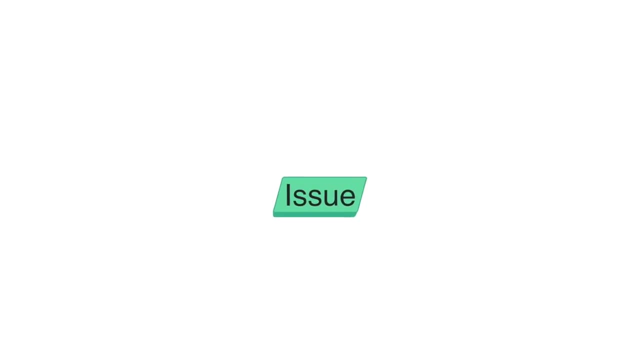 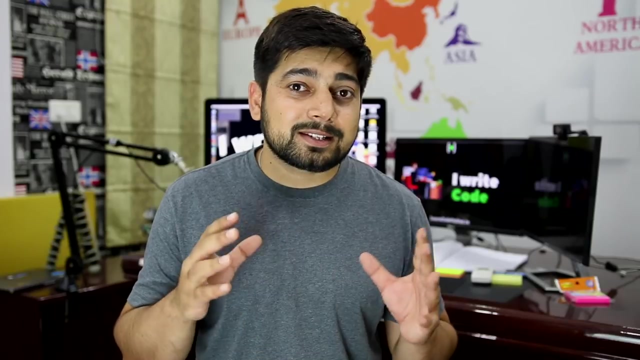 databases are all amazing, but there is one, one big problem with them, which is scalability. Now, if you'll ask any database administrator who has been working with the relational, he'll say that it's all amazing until and unless our company felt a need of scalability. Yes, surely we can. 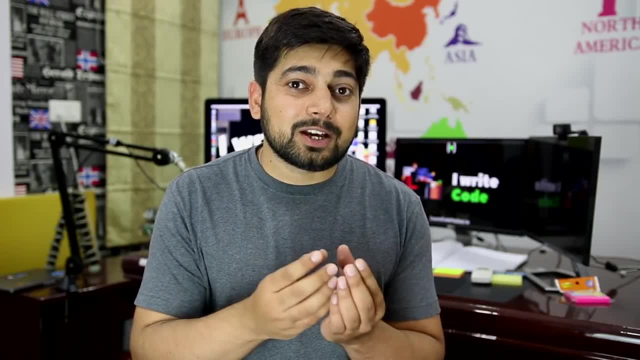 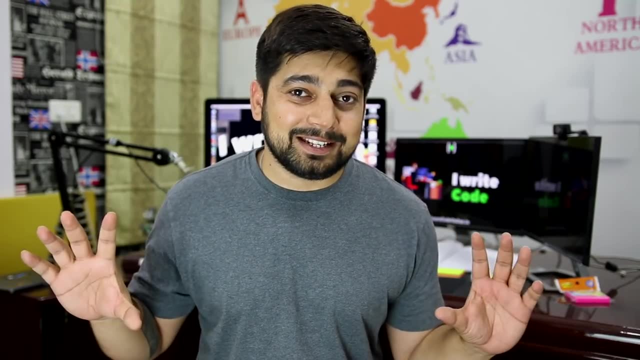 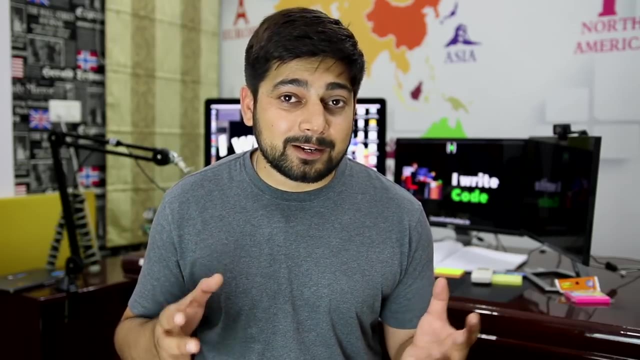 apply more hardware. but that's not the point. We want a scalability in a horizontal level, and these NoSQL databases can be scaled on a horizontal scale. Now, if you'll ask me the difference between the NoSQL and the relational databases, it's actually not that complicated. It's far more easier In the NoSQL databases we focus on. 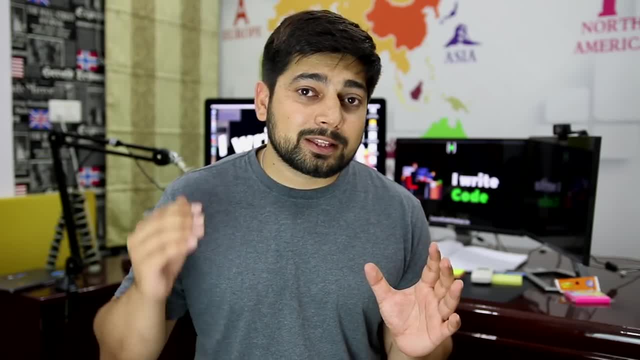 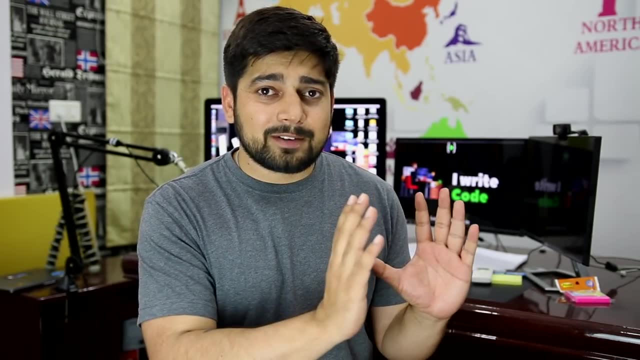 a predetermined structure, known as schema, where all the data or the properties or whatever the value that is is going to come into the databases. We follow that already. we have defined a structure. this is what it comes here. If any other data comes up, we have no place actually to. 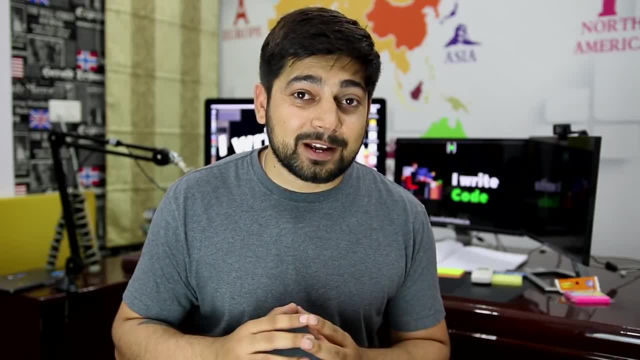 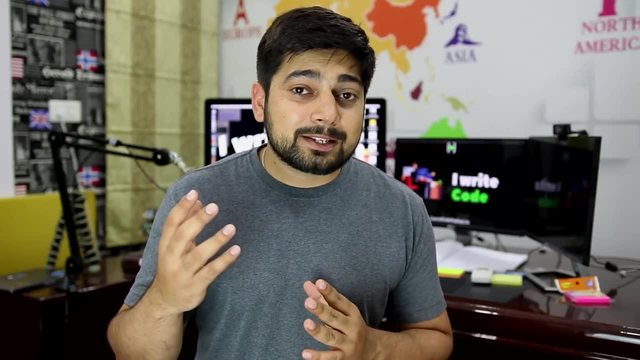 store that data and in some application, that's exactly what we are expecting. This schema is a formal definition of how data is going to be structured and is going to be stored At some places. we expect that it should come as an integer. It should always come as an integer, and there is 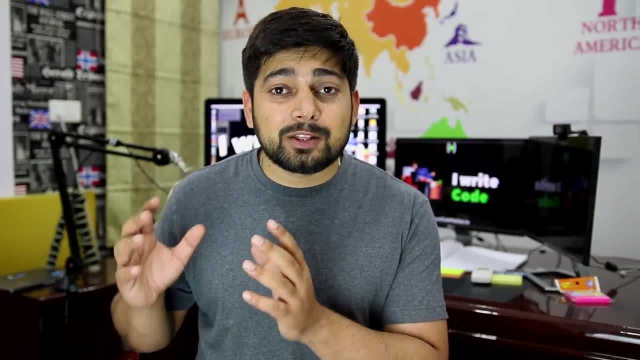 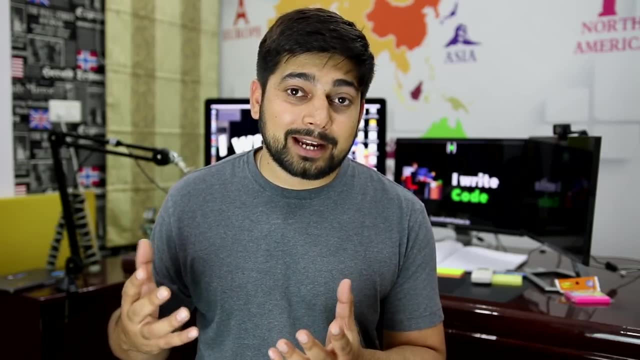 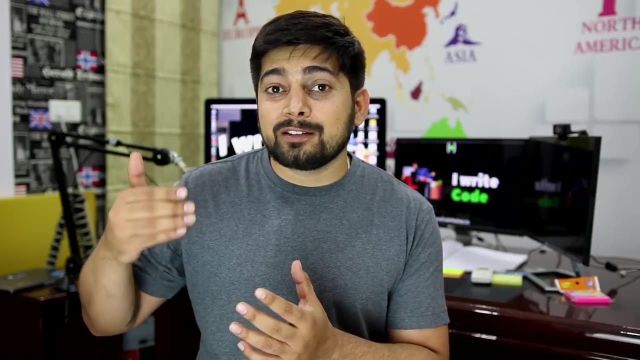 no exception for that, While, on the other hand, if I talk about the NoSQL databases, in NoSQL database, the data is structured and is stored in a freeform format. Now, this freeform format can be simply like a JSON format, but don't pick the word here, because it can be stored in variety of other formats as well. 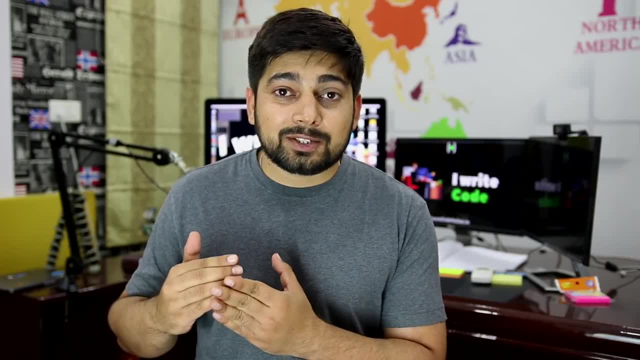 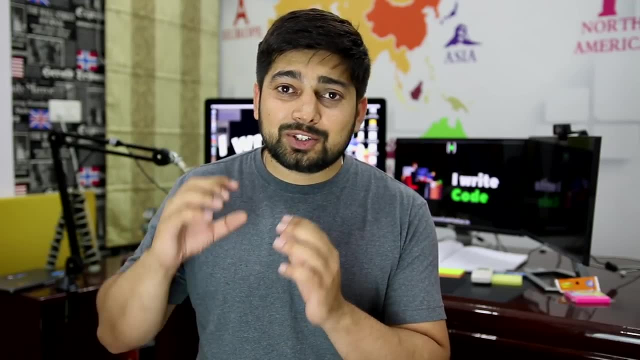 JSON is the most common one Now in the NoSQL databases. even if the data which you are not expecting is going to come up, you don't need to rewrite the entire structure. you can eventually, just at that point and at that moment, you can go ahead and store that data. Okay, so that's the most. 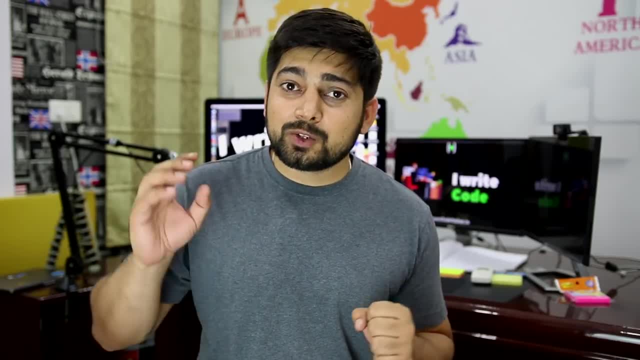 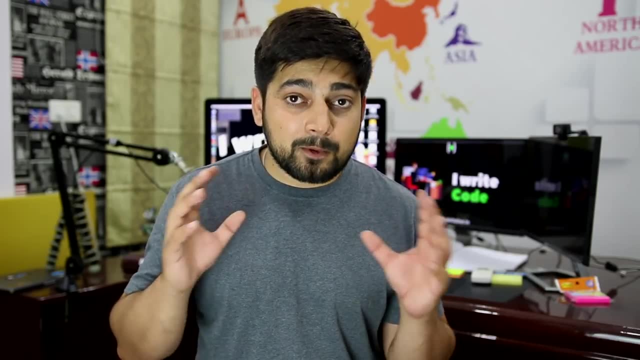 common and fundamental thing that you need to know about the NoSQL. So what are the more things that you should know about the NoSQL databases? Now, NoSQL databases are basically just a bunch of categories that you can categorize into four categories. You can see that the NoSQL databases 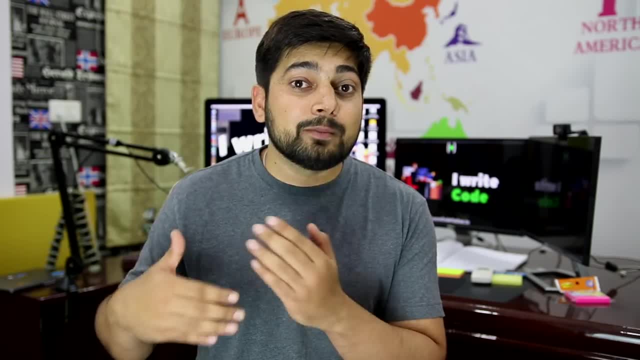 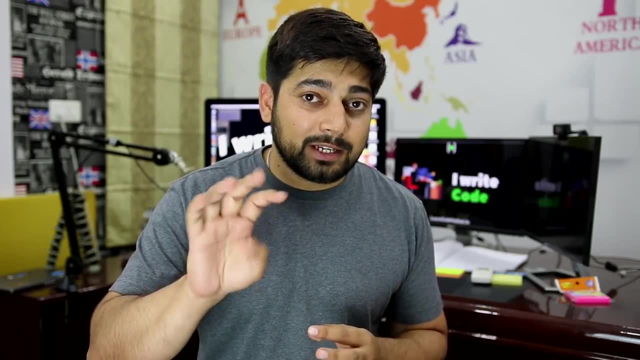 are categorized broadly in four categories, but hey again some of the books and some of the reference point, you'll see that there are even more categories. but the whole fundamental, whole core point of these NoSQL is divided into four categories. The first and the most common one, 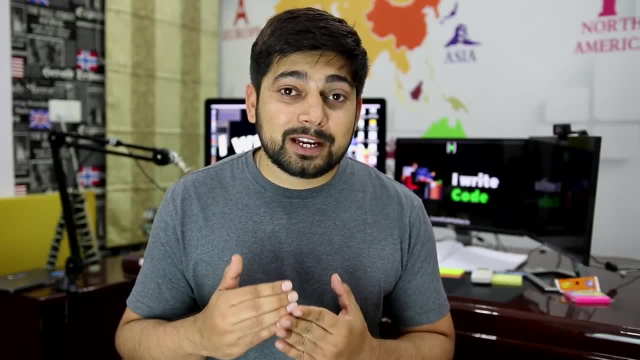 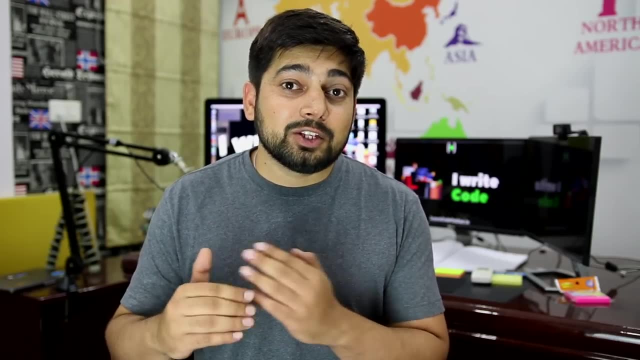 among all these categories is document database. The example could be MongoDB, which is my personal favorite. In these kind of database, you just collect the entire data that you want to store. The entire structure is in JSON format, Even if the new data comes up. you just create a new object and that is stored in a whole. 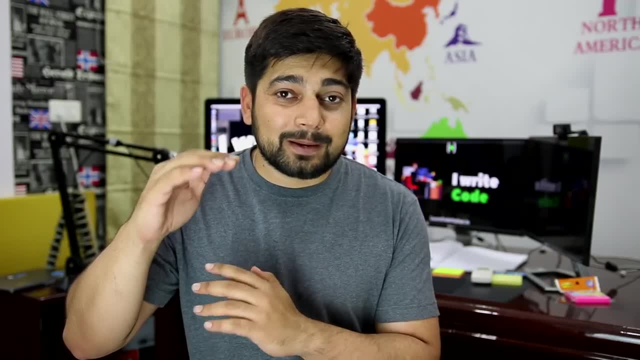 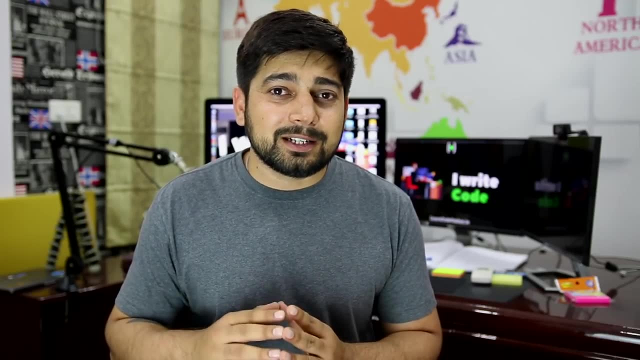 gigantic, big object, Really the fun one to work with them. very easy to understand their structure, very few queries that you have to like, learn and all these things. very small learning curve, and these are kind of my personal favorite one Now, next up in this category is a key value. 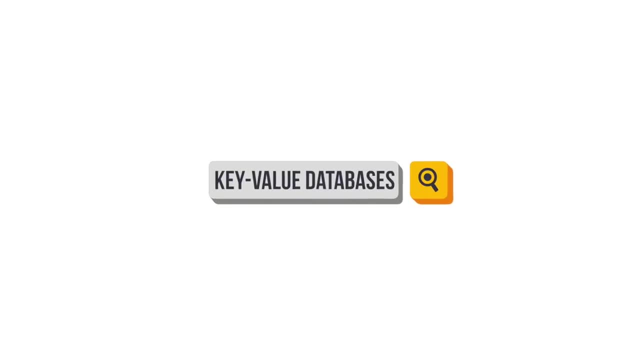 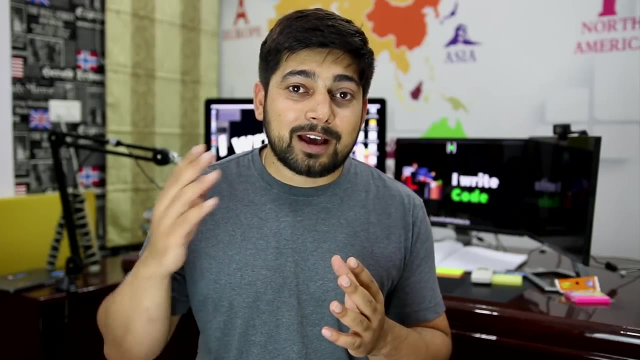 database. Now, there can be other names for that as well, but the whole idea is everything in this kind of database is stored in key value pair. Whenever you want to access something, you just mention your key and your value will be produced. The example could: 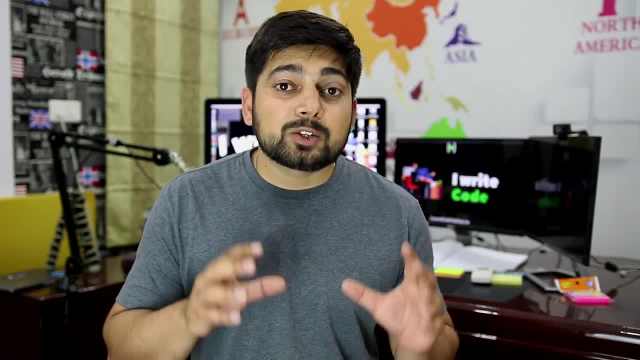 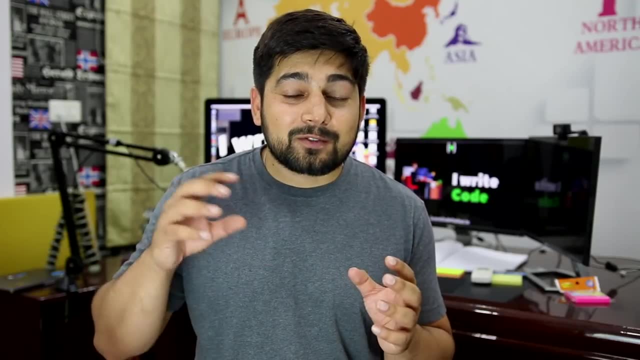 be like Redis database. Next up, the third category is wide column database. Now, in this there's a strange thing that happens: everything is stored in columns instead of rows. that we are kind of familiar with. the relational databases Now the example could be Cassandra, and these are one of 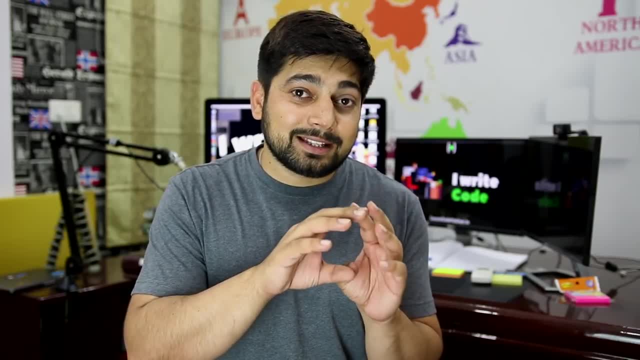 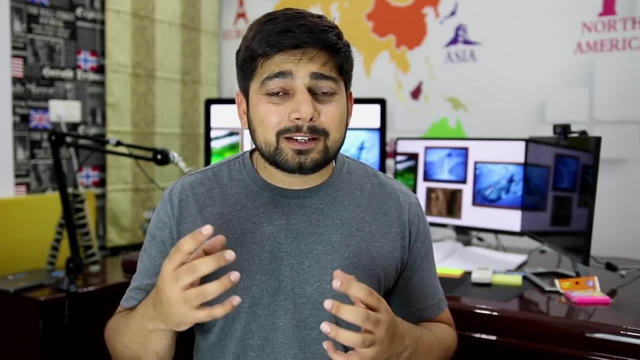 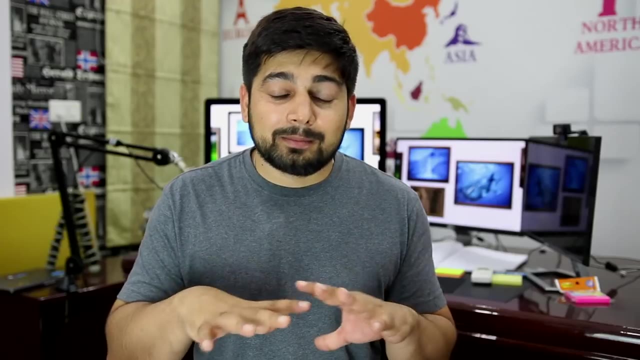 the most powerful ones because they can store anything in column and at this this can be actually scaled horizontally, like endlessly. And the fourth one and last one is little bit complicated at first to understand and it's a node based database structure. Now some call it as a graph database as well, but again, regardless the terminology, the whole point is: 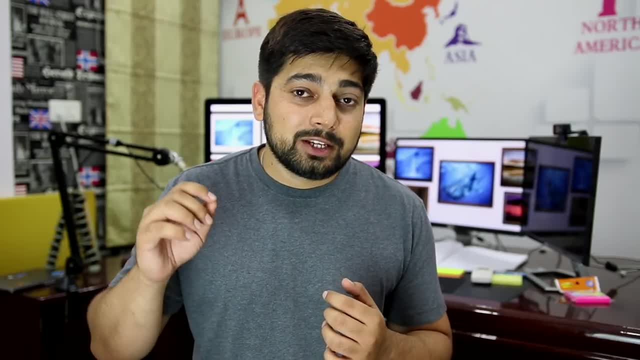 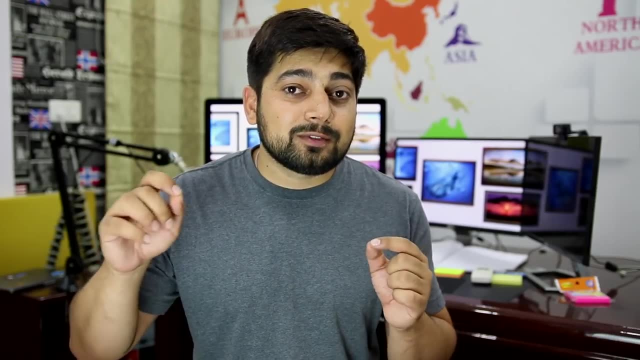 everything is stored in point in the format of a node. Your data is also going to be stored in the format of node, and that node is also going to store your relation with the other points that you want to anchor Now. yes, it's a little bit complicated to understand at first, but one of the 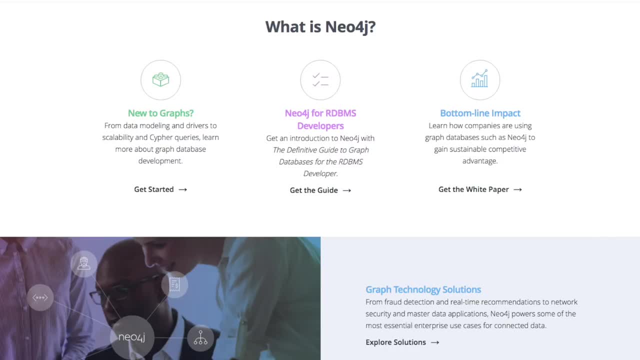 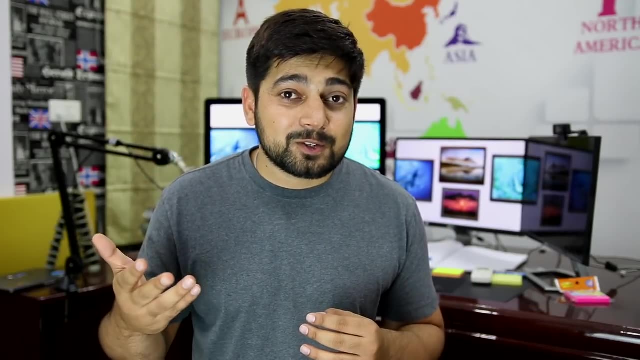 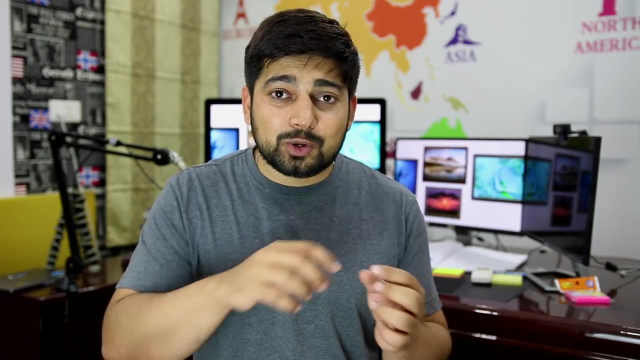 example is Neo4j. Now, these databases, once you understand it can be like really amazing. but also I would like to make a point that these databases like Neo4j is not for a small scale application. These are for somebody like Facebook who has so many endpoints, so many nodes, so many connections with the data. So Neo4j- 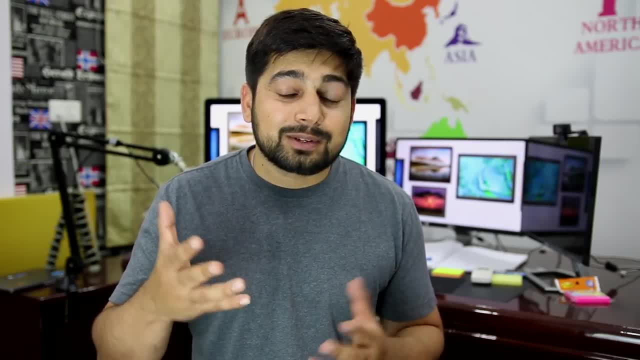 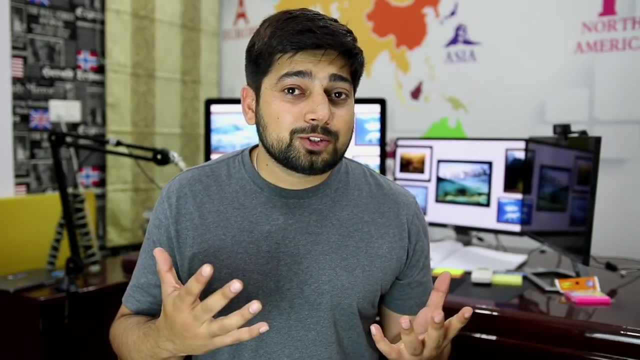 is one of the ideal database that should be used by Facebook, and, of course, it is being used there. Okay, so now that you understand quite a lot about the NoSQL, the obvious question is when you should be using NoSQL and when you should be using relational databases. Now for most of the small scale. 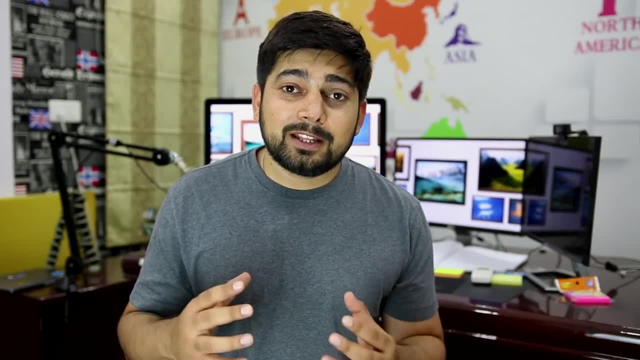 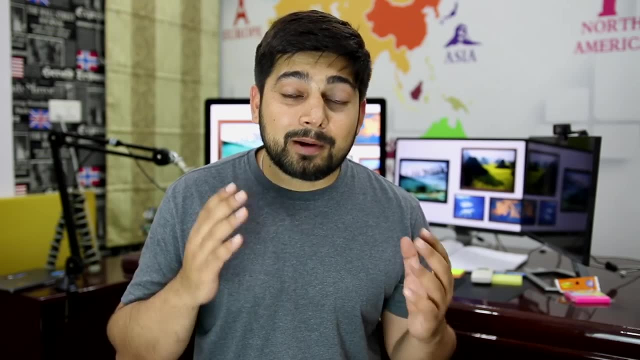 applications. still, the relational database is amazing, but when it comes to your startup, whatever you are trying to design, or your product- now, it comes to a variety of things- Companies spend months and months to decide what is going to be the stack of their technology, because it's not. about the favoritism. It can be not about, like: my favorite is java, his favorite is javascript and his favorite is swift, so we are going to use all of them. No, it's not about that. At the end, business decision are based on money and how easily you can find developers for them. So companies do spend. 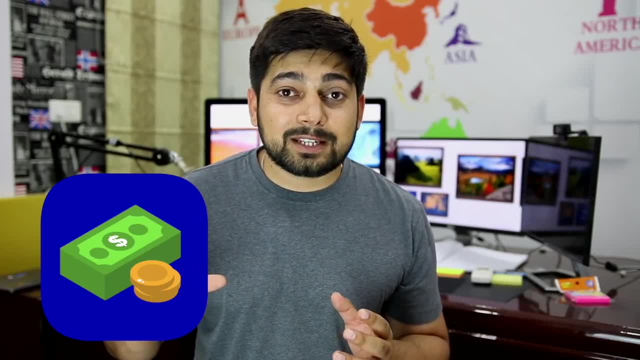 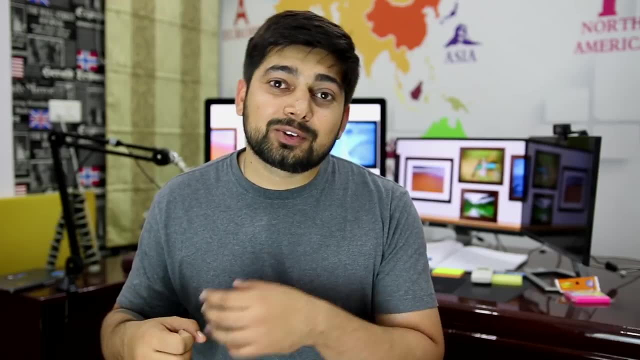 a lot of time in that. Now, once they have decided that this is going to be our stack and all the research goes good for the NoSQL and their purpose, then only it is decided that it's going to be NoSQL or maybe relational databases. Now, usually when the companies are much more worried about 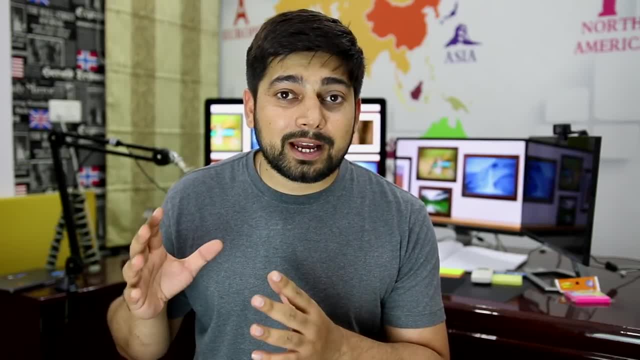 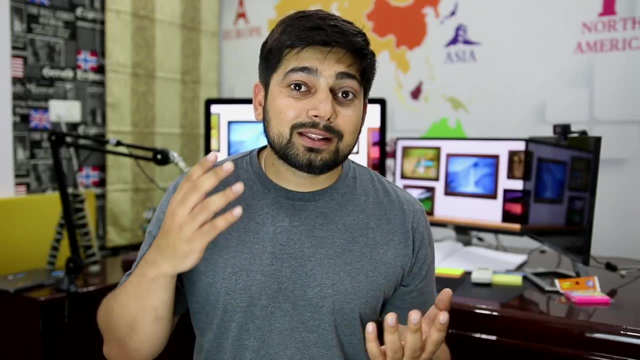 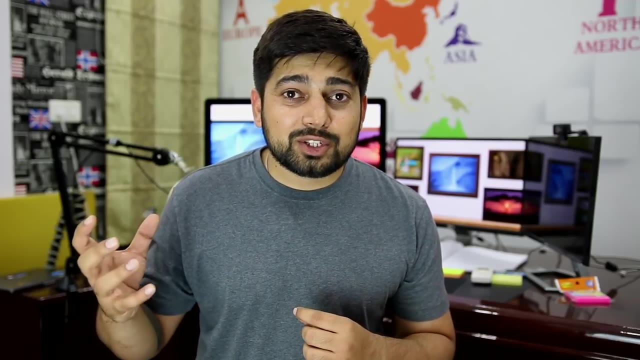 the fast access of their data and how the structure is going to be laid. this is the main point when they decide whether it's going to be NoSQL or relational. Remember that MySQL- the relational databases, are still faster, but again, when you compare the speed with small transactions, NoSQL proves to be a little bit more faster side when you have fast. 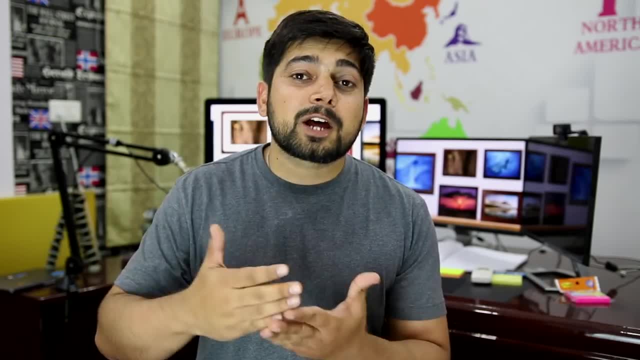 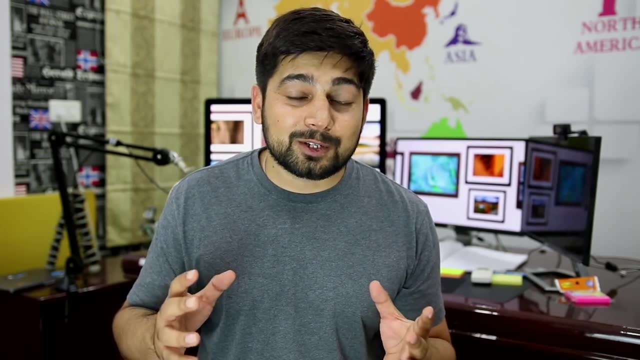 access and flexibility of the data. Or maybe your startup or your company is looking forward for the scalability solution. You know, you are pretty sure that you will have plethora of users and eventually scalability could be a nightmare for you. That is one of the point where you decide. 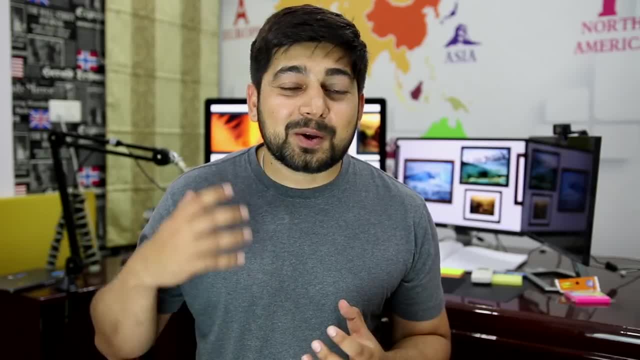 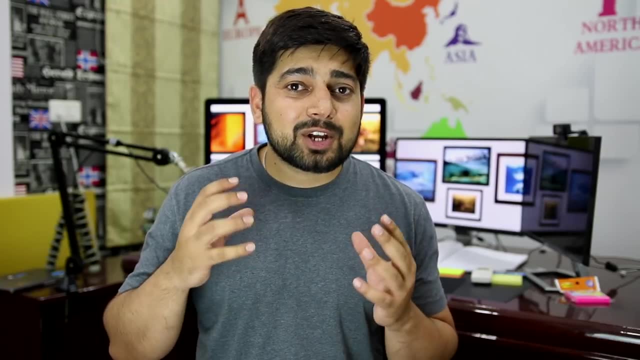 that, hey, I'm going to go for that. Okay, so now you know quite a lot about the NoSQL. The obvious question that might be pondering in your mind is that in the NoSQL we get such a high speed when we want to access the data? 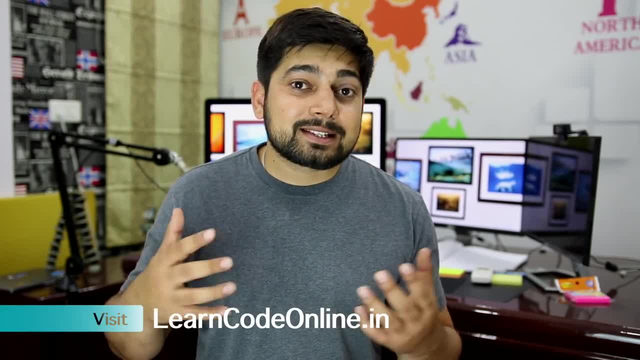 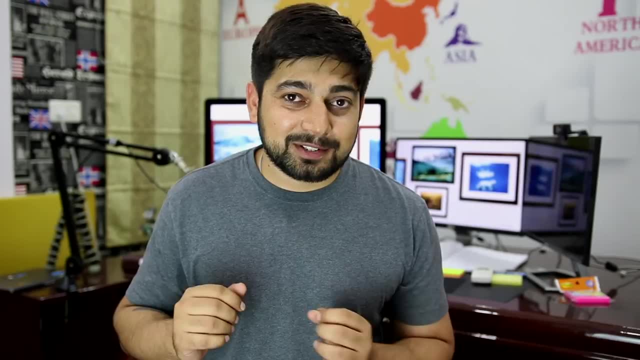 We get the flexibility of storing the data as well. Plus, the scalability is amazing. So why don't we just use NoSQL everywhere and just abandon these relational databases? That's actually a good question Now. actually, all of these points are correct and at some point of degree you are right. 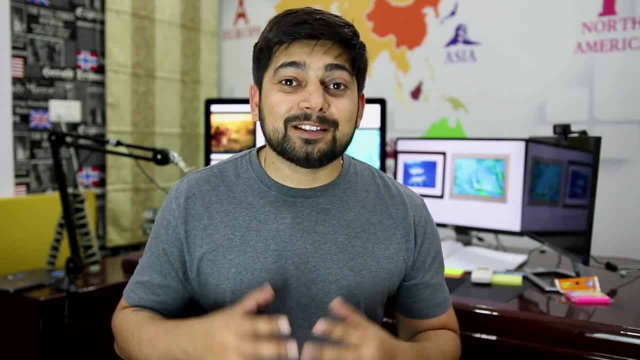 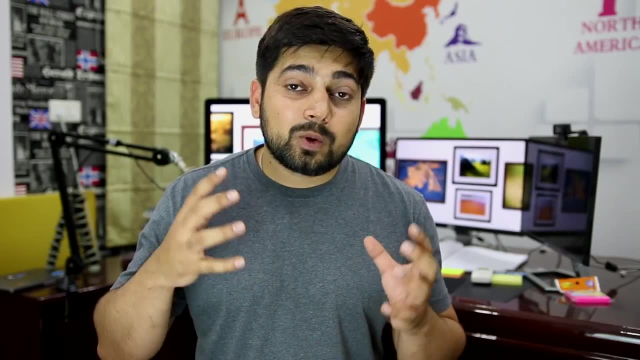 and you will be able to use NoSQL. But let me tell you one thing: Not everything in this life and this world is all sunshine and rainbow. Things always come with their limitation, with their pros and cons. And what are the advantages here in the NoSQL are actually its downside as well. 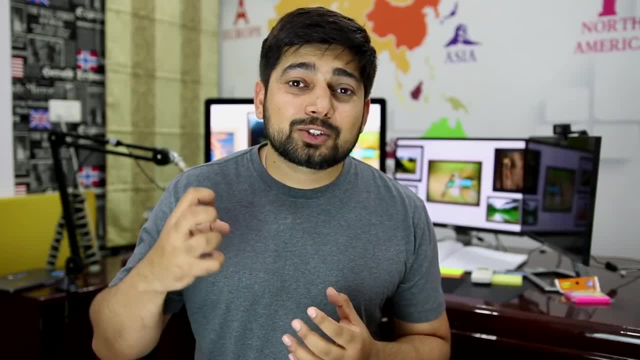 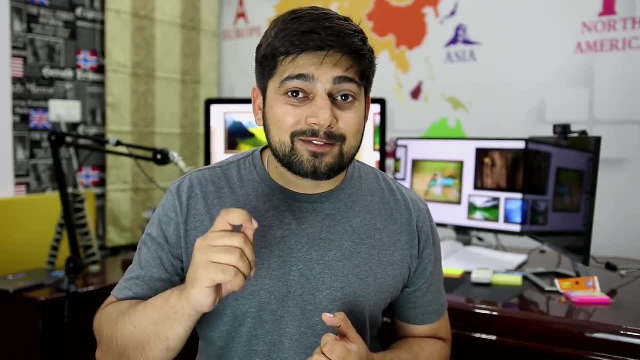 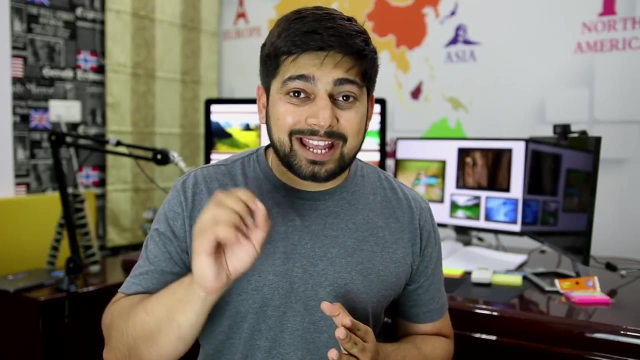 There are still many such applications which are so complex as well as so, and require so much of the constraints about these transactions and their reliability on the transaction and their safeguards, that relational databases are much more complex. Now, of course, NoSQL is all amazing, but the whole property, the asset property, 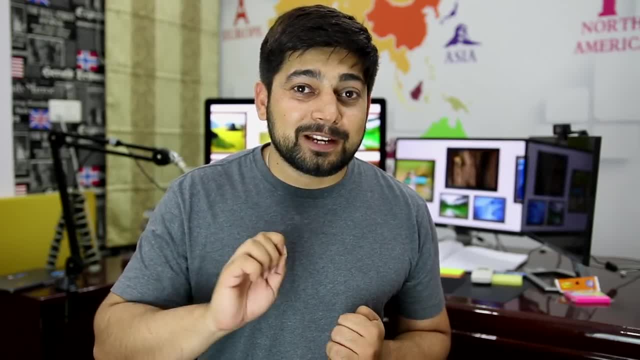 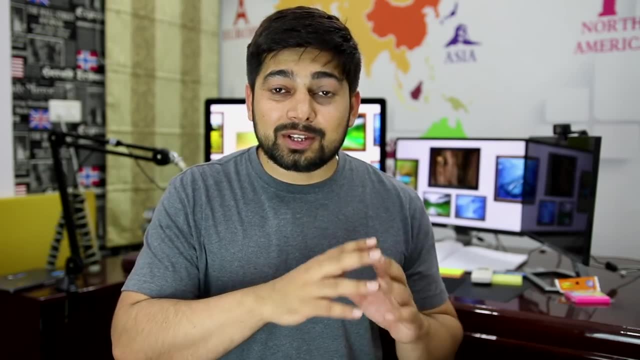 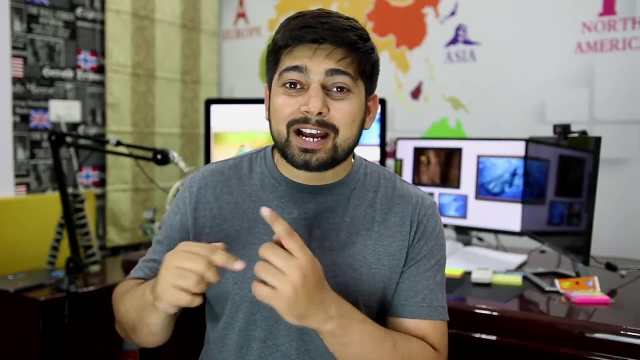 I highly recommend you to google a little bit about the asset property of databases. Now these asset properties are compromised a little bit in the NoSQL, While the relational databases, they, are whole rigid about that. So eventually these compromises in the asset property are actually the.